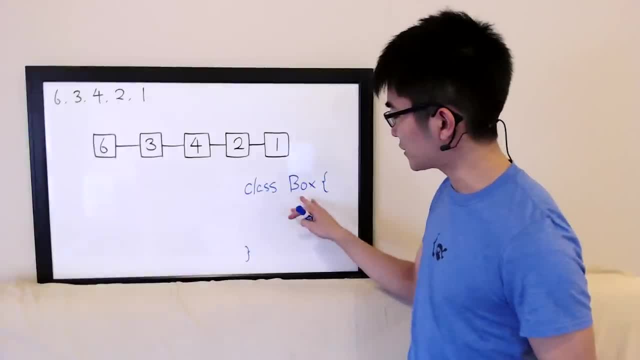 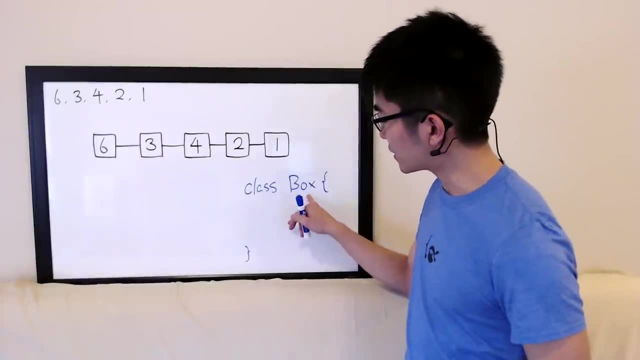 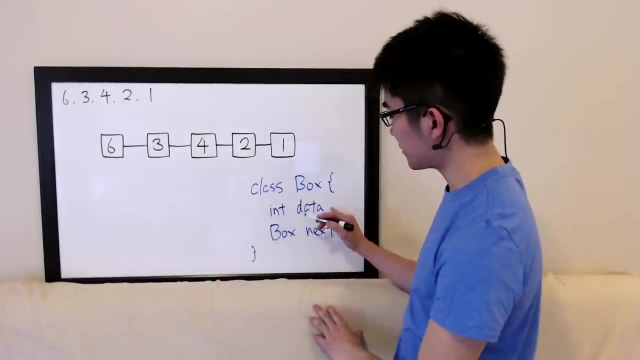 object and let's say the class for that object is called box- actually, we'll rename it later, we're going to change the name later, but let's for now call it box- and it's going to have two attributes or two fields in this class and the first one of those attributes is going to be called data. 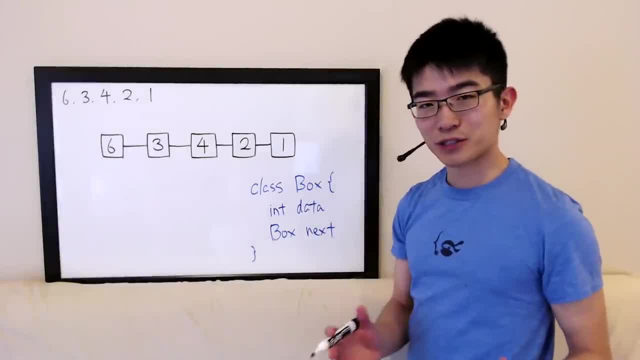 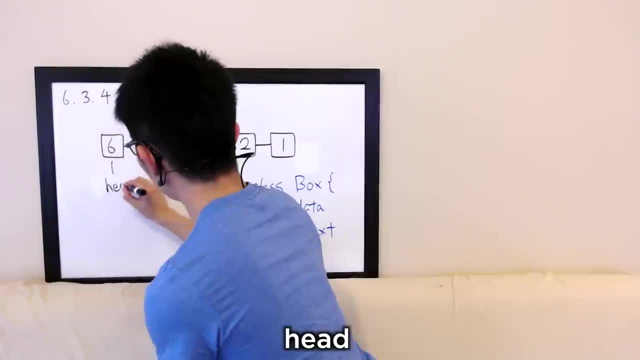 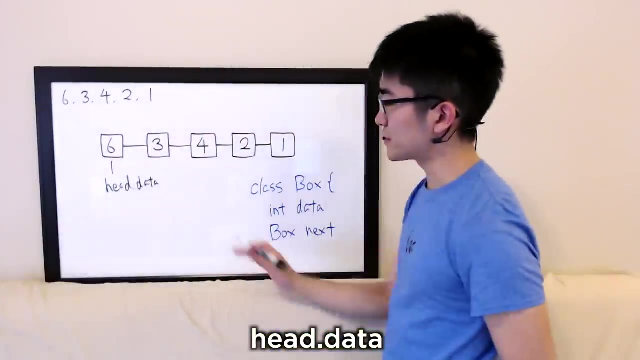 it's going to be the data or the item each box contains. so if you have, let's say, the first box in a variable called head, if you write head dot data, that's going to give us this value six right there, because that's the data head the first box contains and the type of data could actually be. 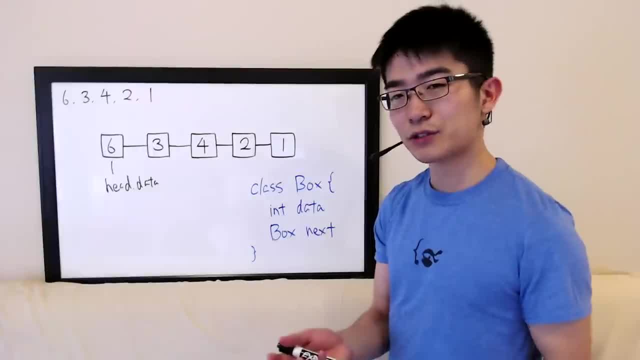 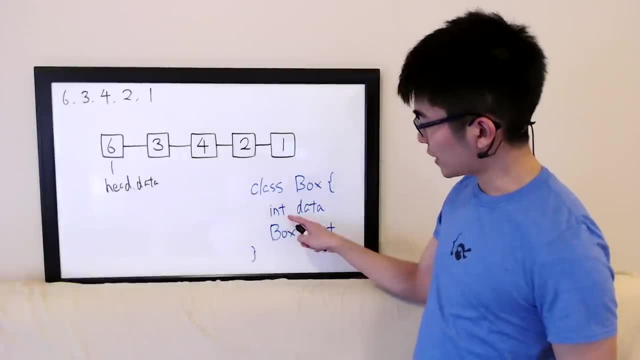 anything. it could be an integer, it could be a string, a character or anything else for that matter, but here i'm just assuming that it's an integer, just for simplicity, and that's why i wrote int data here and the second attribute here, or the second attribute here, is going to be the item each box contains and the second attribute here. 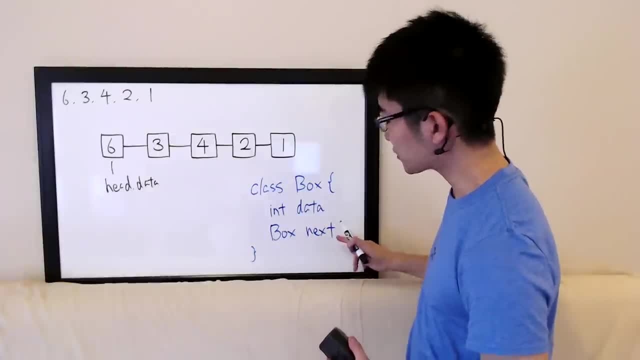 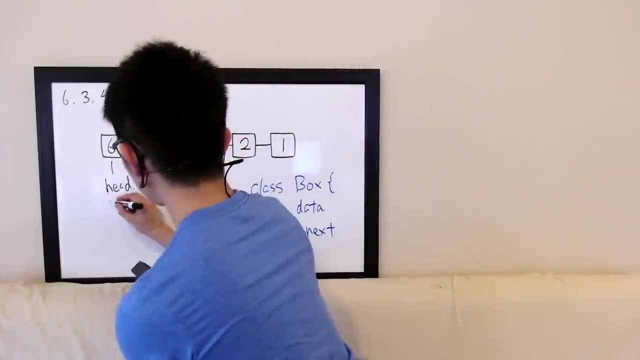 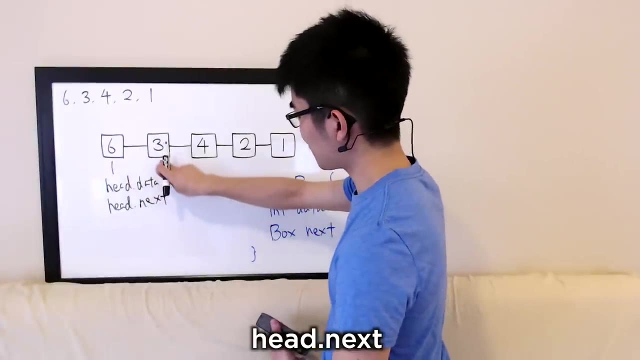 or the second field is going to be called next and that's going to refer to the next box that's connected to that particular box. so if you write head dot next, that's going to refer to the next box, to this box head, so that's this box right here. and so if you write head dot next, dot data. 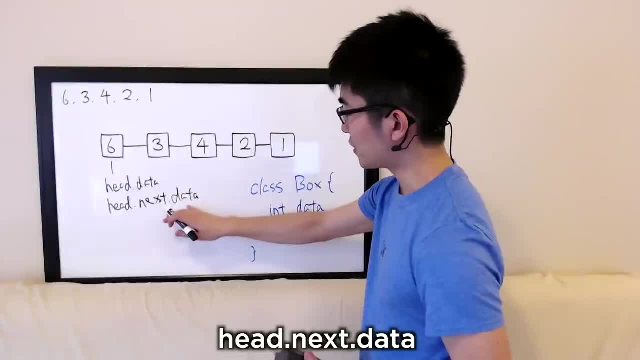 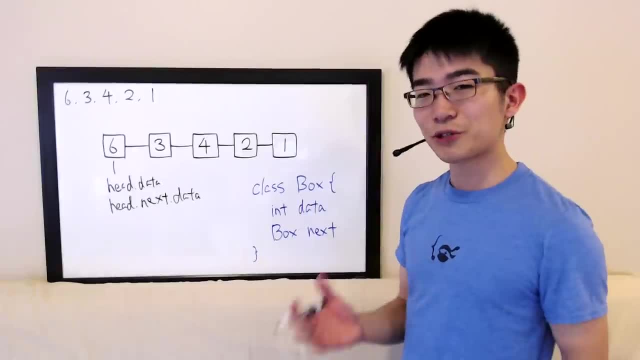 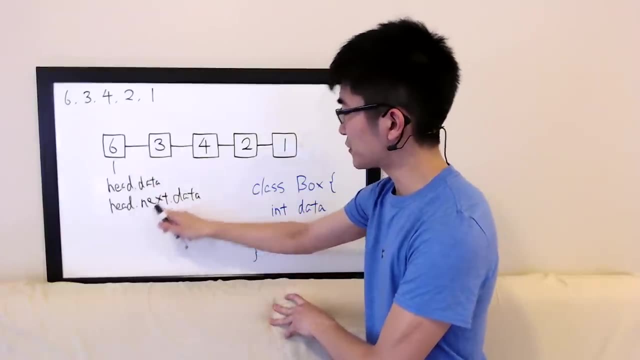 that's referring to the data attribute of the next box of head. so that's the number three right here. so just for clarity, head refers to, of course, the first box right here, and then head dot. next refers to the next box, this box right here, and then head dot. next dot. data. 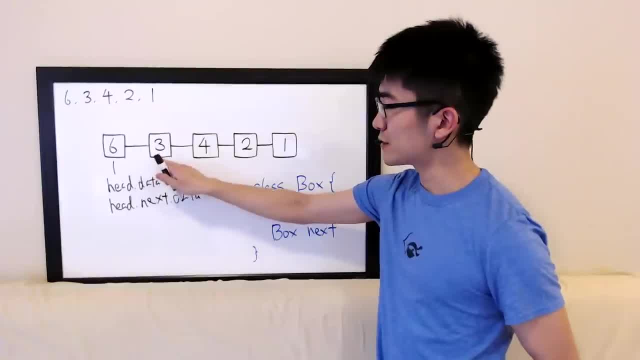 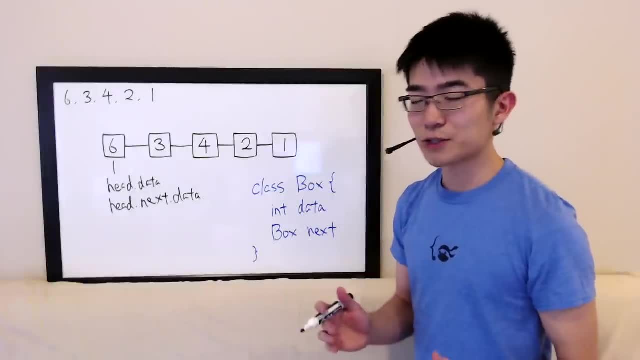 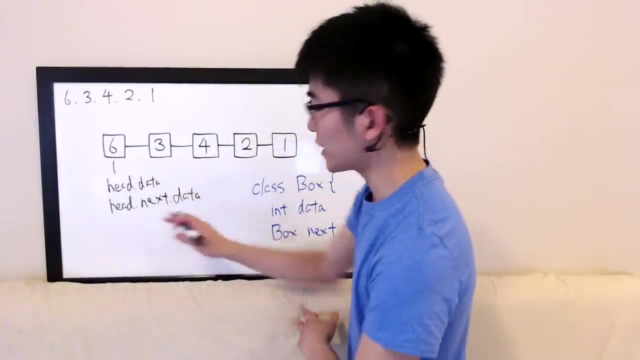 refers to the data inside this box. that's number three right here. okay, so once you have a reference to a particular box, or once you have a variable containing, let's say, the first box right here, head, you'll be able to find the next box, of course, by writing head, dot next, and then you'll be able to find the next box after. 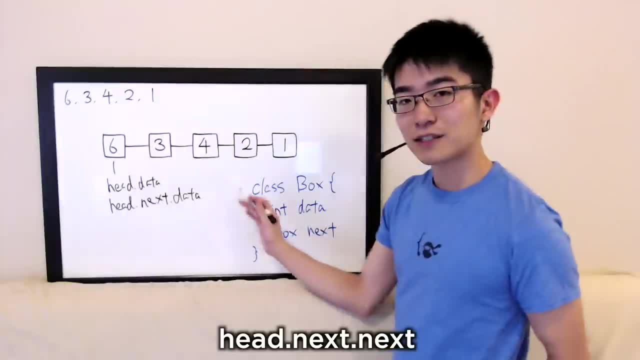 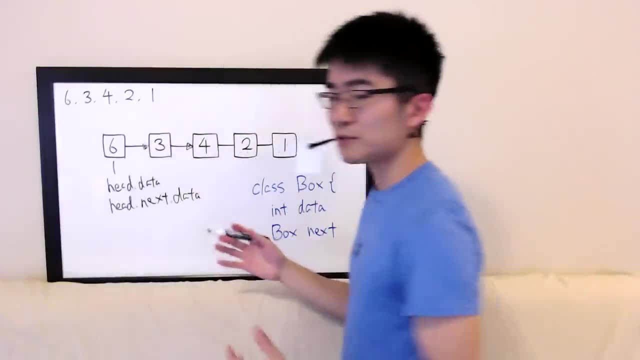 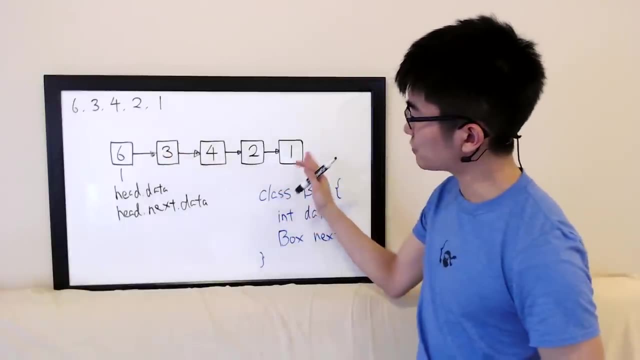 that this one, by writing head: dot next, dot next. so you can go from left to right in this diagram very easily, but you won't be able to go from right to left, and that's because in a link list these connections go in one direction but not the other way around. so if you have, let's say, this middle box, 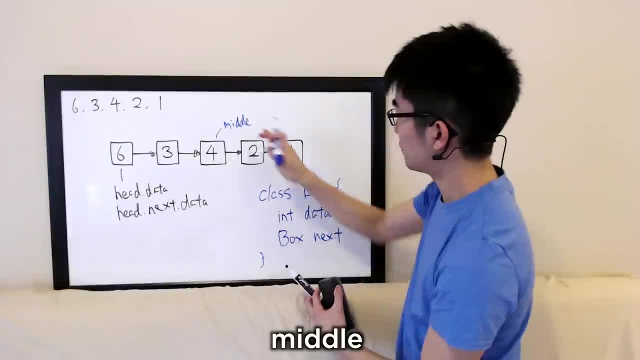 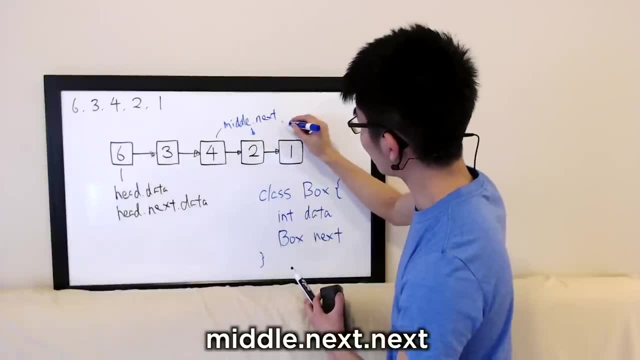 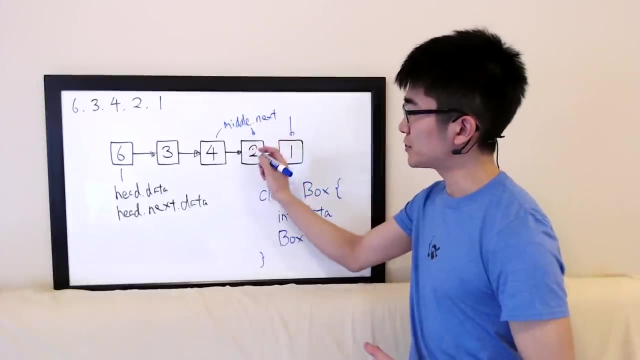 right here, and and and. a variable called middle, middle dot next will refer to this box right here. and then middle dot next, dot next will refer to this box right here. but if you want to somehow use the middle variable to find the previous box that contains number three right here, there's no easy way to do that. 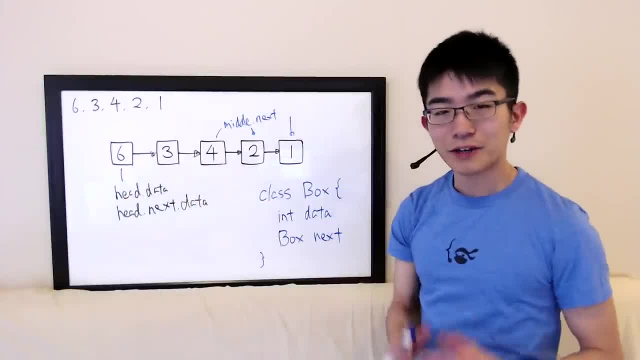 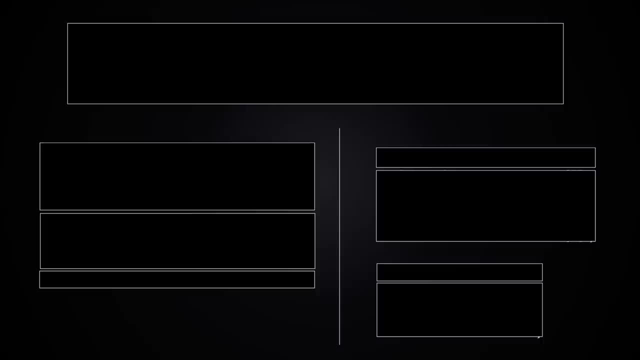 unless you start from the very beginning. okay, so that's the basics of how link lists work, and let's see how you can actually implement the link list in a very simple way. so let's start with the first box and then we're going to implement it using code. here, let's say, as an example, we're trying to create: 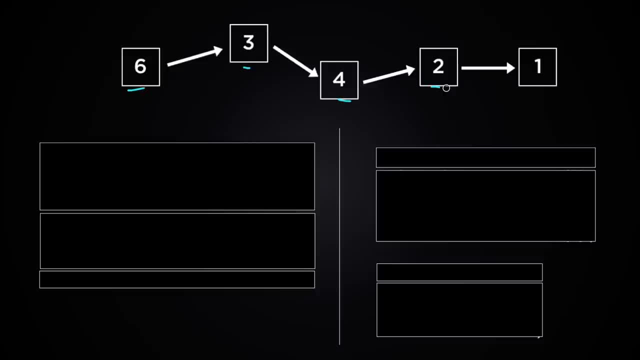 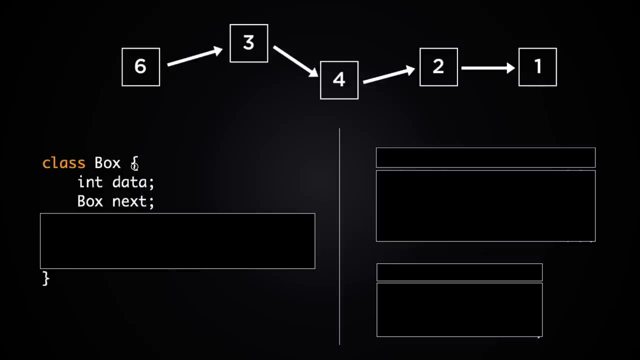 this link list with the numbers six, three, four, two and one, and here we're going to take a look at some code in java as an example- but other languages are going to be pretty similar- and in java you can define a class called box just by writing class box, curly brackets, and then it's going to. 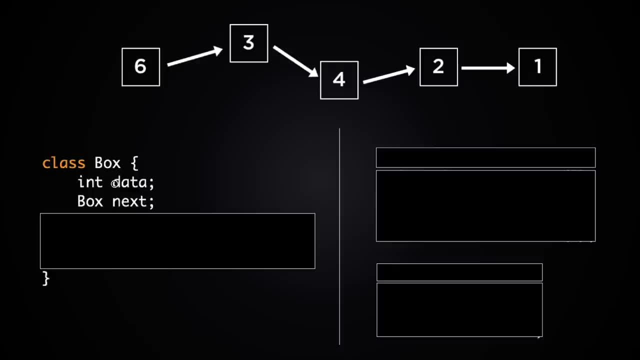 have two attributes or two instance variables, like we saw earlier. the first one is data, which is an integer, and the second one is next, which is going to be a box. so this is actually pretty much all we need, but to make our lives slightly easier, let's define a constructor too. this is going to 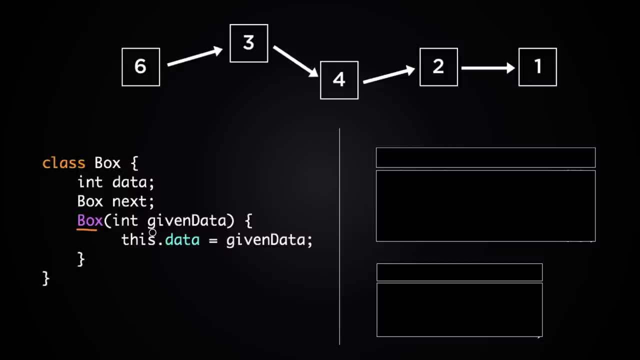 be called box, of course, and it's going to take given data, which is an integer, and then it's going to set that new objects data to given data. so with this constructor, if you write new box 6, for example, you can create this object right here and then you can create this object right here, and then you can. 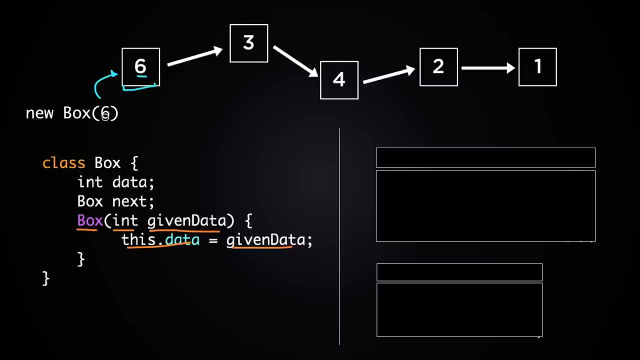 create this object right here, a box that contains six as its data, and when you create a new object with this constructor, the next attribute of the object will be set to null by default, and, of course, now just means that there's nothing there, and the common convention here is to make the argument. 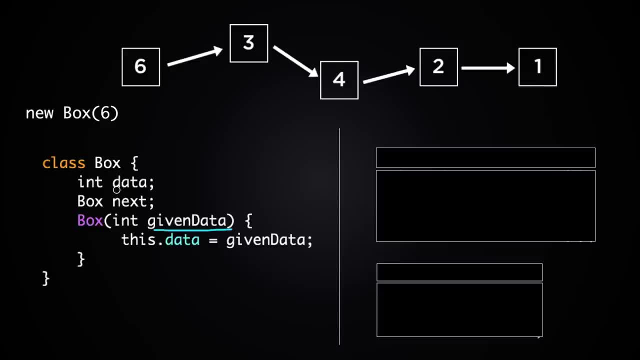 name here, given data, the same as the attribute name data. so we're going to rename given data to data. okay, so we now have the same code here as before, except for the fact that in the constructor we renamed the argument name to data from given data. and another thing is: when people make link lists, 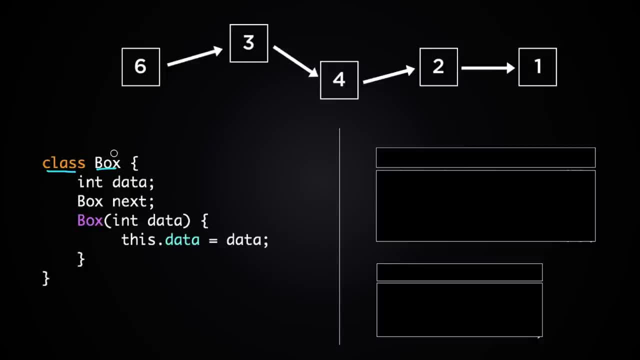 they usually don't call this class box. instead, they usually call it node. so let's rename this from box to node. okay, we just renamed it and here we have node instead of box, but the idea of the code is exactly the same. so let's rename this from box to node. okay, we just renamed it and here we have node instead of box, but the idea of the code is exactly the same. 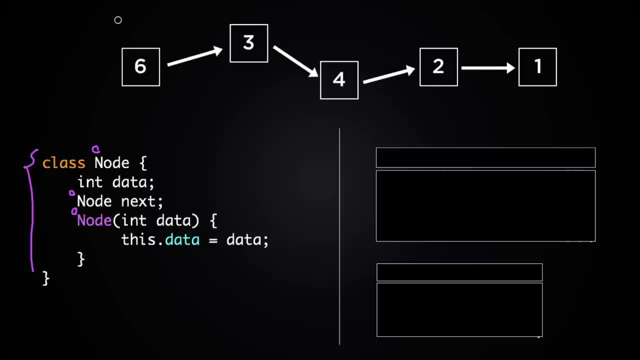 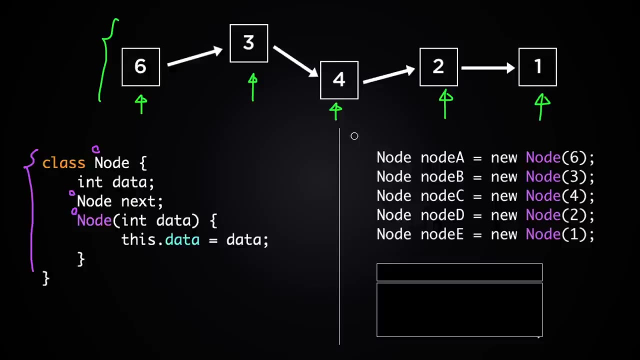 and let's now think about how we can create this particular link list. the first thing we want to do is we want to make these five boxes, create these five boxes or five nodes, and we can do that with code like this: if you look at the first line here, we're creating a new node with the data six. 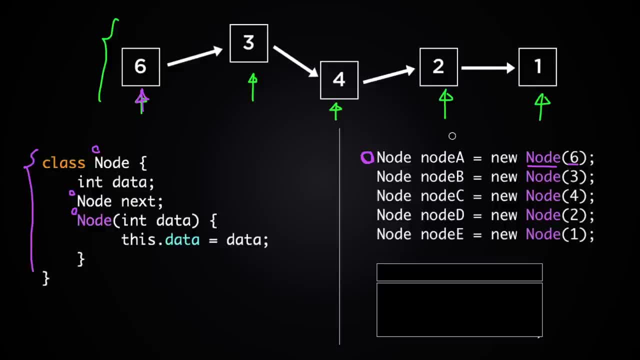 so that corresponds to this box right here, and then we're assigning it to a variable called node a, and then we're doing the same thing for the four other nodes, just by saying node b equals new node three, and so on. so after executing this block of code, node a will be this one, right here. 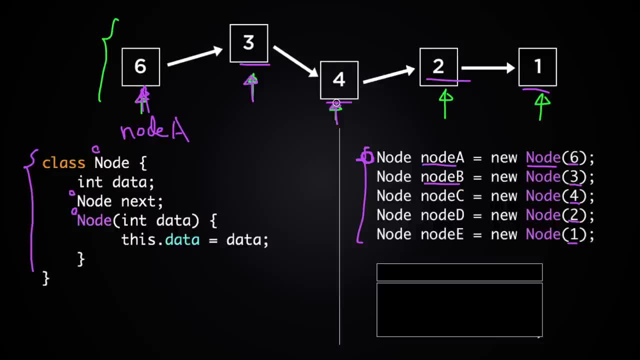 and then node b will be this one right here, and then c and so on. but if you only had this block of code, these boxes, these nodes won't be connected to each other. and that's just because when you create each of these nodes with this constructor, the next attribute of each of these nodes will be: 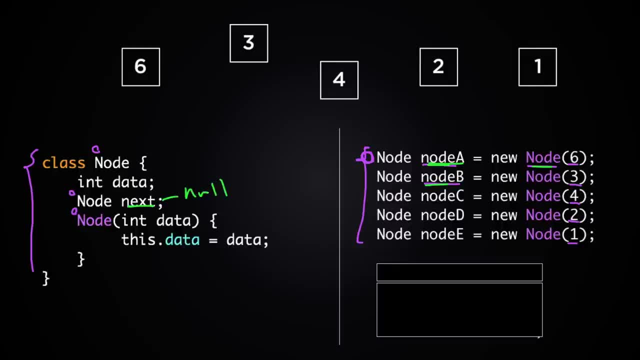 just null or nothing. and we can fix that just by writing something like this: this line right here, node a dot next equals node b. sets the next attribute of node a. this one right here to node b. this one right here. so it's sort of like drawing a new arrow here from node a to node b. 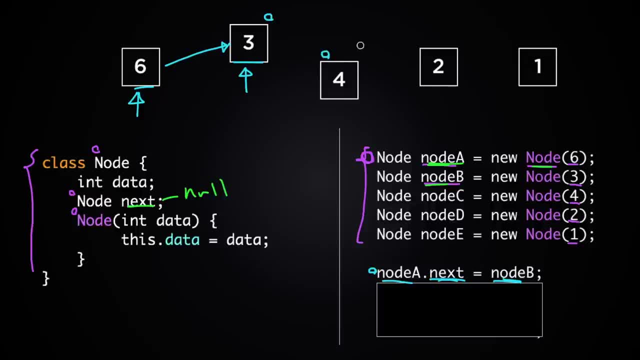 and we can do the same thing for every other pair of nodes that we want to connect, just by writing this. here we have node b, dot. next equals node c. so this is saying the next attribute of node b, this one right here, should be node c, this one. 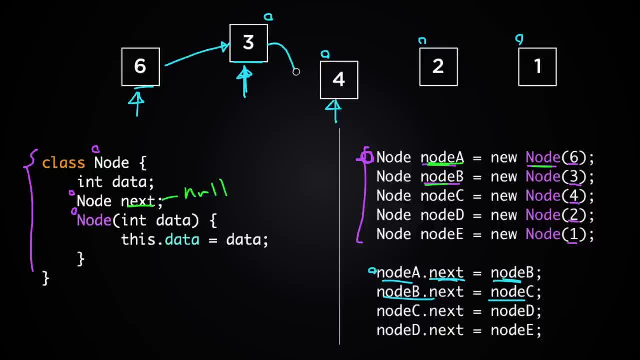 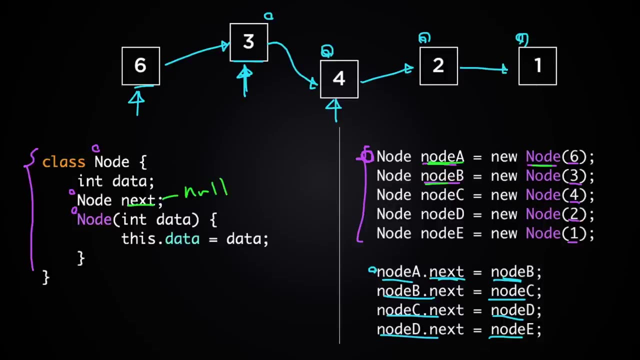 right here. so that's like drawing an arrow from here to here and we're doing the same thing for every other pair by writing: node c- dot next equals node b- this one right here. and then node d- next equals node e- this arrow right here. so this method of creating a new link list works just fine. 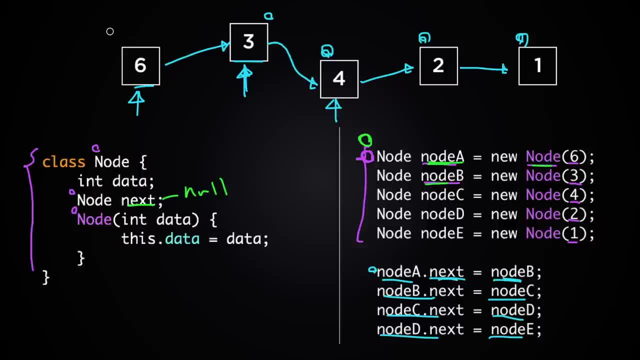 but it's pretty awkward because whenever you want to create a new link list with this method, you need to create these nodes manually and then connect those nodes manually as well. and if you want to avoid doing all that manual work, one way to do that would be to create a new class called 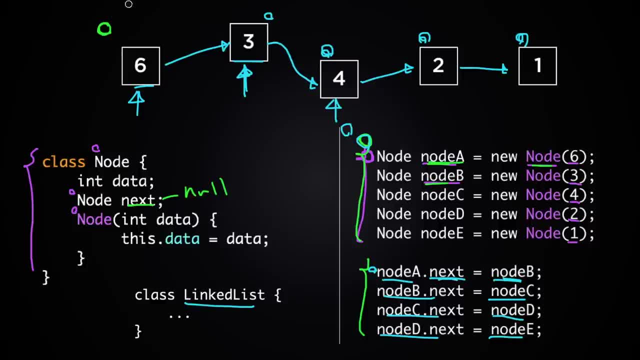 let's say link list, and then whenever you want to create a new link list, you can just create a new link list object and then have that link list object contain all of these nodes inside. so, visually speaking, it's sort of like creating a new link list object and have that object. 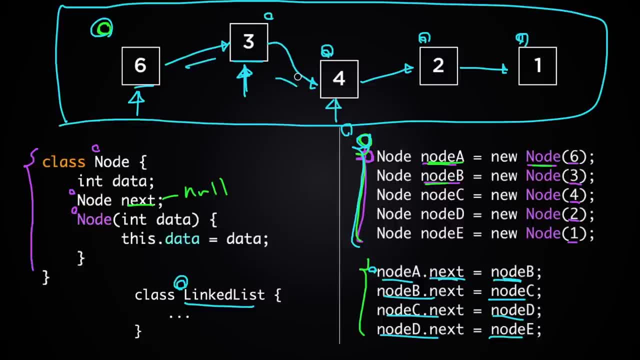 contain all of these nodes and these connections inside, and then within this class you can add functionalities like, let's say, add a node which automatically adds and creates a new node for you, and that function could also create a new connection for you, for example this one right here, and then you can add other functionalities to this. 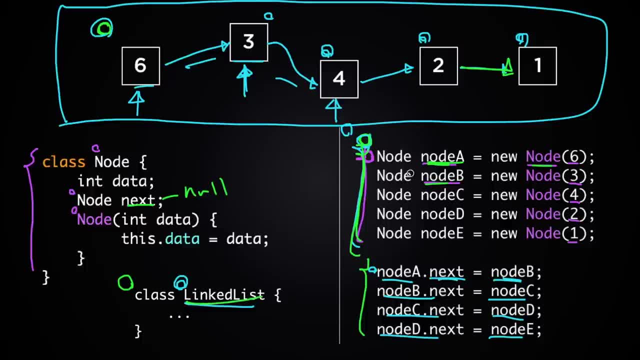 class as well to make it even more convenient. like, let's say, delete node which deletes certain nodes for you and maybe find a node which finds a node with a certain value. so that would definitely be one good way to simplify this whole block of code using a class. 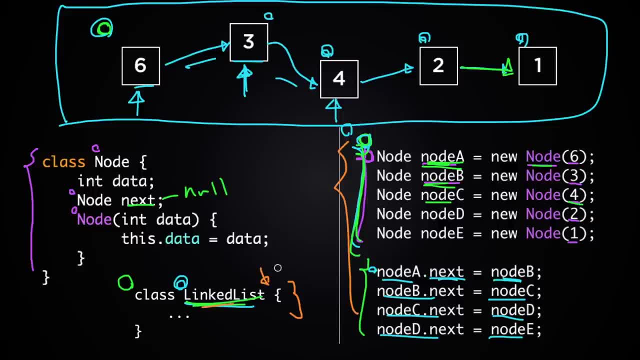 but instead of diving into how to define and implement this link list class, i'm just going to give you sort of a practice problem to help you better understand the concepts i explained so far. and here's the practice problem. let me just quickly explain the setup. first, you're given a 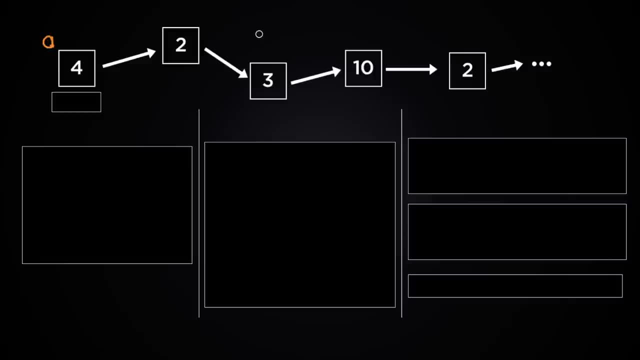 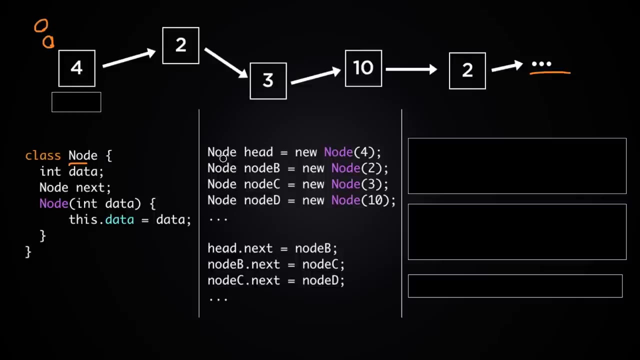 link list that might look like this. and then let's say, you don't necessarily know how many nodes are there in this link list, and this link list is based on the same class that we saw earlier class and of course, this link list might have been created with code like this. so we're defining 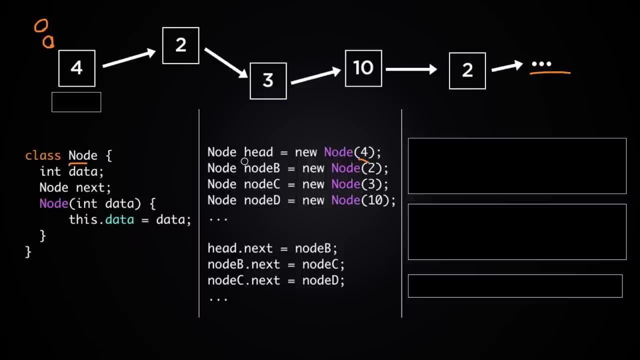 a new node, of course, with the value 4, and then that node is going to be set to this variable head, right here. and then node b will be a node with the value 2, so that's right here. and node c will have data 3 and so on. and here we're making those connections, those arrows. so head dot next. 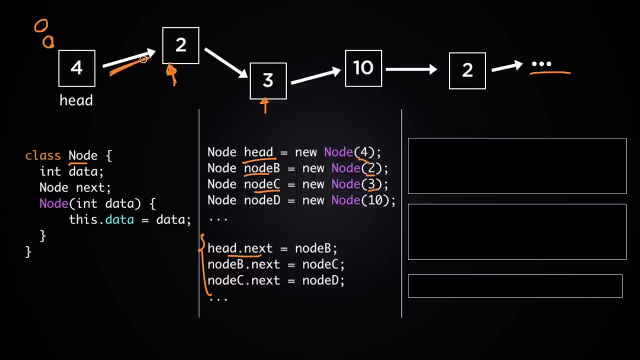 equals node B right here. So that's this arrow right here. And then node B dot. next is node C, So node B is this one, node C is this one, So that line represents this arrow right here, and so on, And again we don't know how many nodes we have. 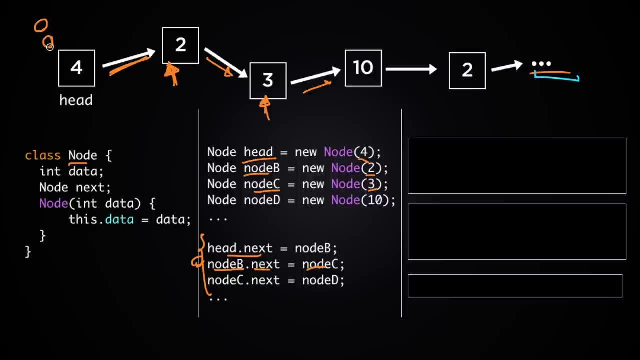 in this linked list. but here let's assume that this whole structure has a regular linked list structure, meaning we have a node at the beginning here and then it's connected to another node and to another node and so on, And these arrows only go in one direction. 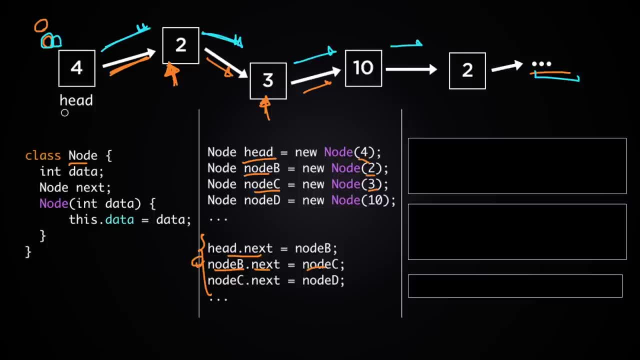 but not the other direction. Okay, so the problem here is: given this head node, this head variable, can you write a function that takes this head variable and then returns the number of nodes in this whole linked list? So if you wanna use Java to solve this problem, 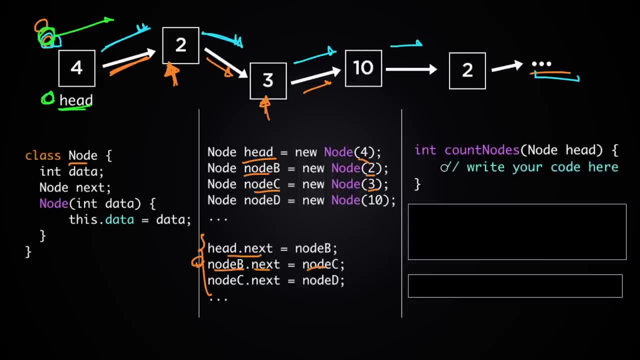 your function header might look like this: Here we have a function called countNodes which is going to take the head node that could be this head node right here, and then it's gonna return an integer which is going to be the number of nodes in this linked list. 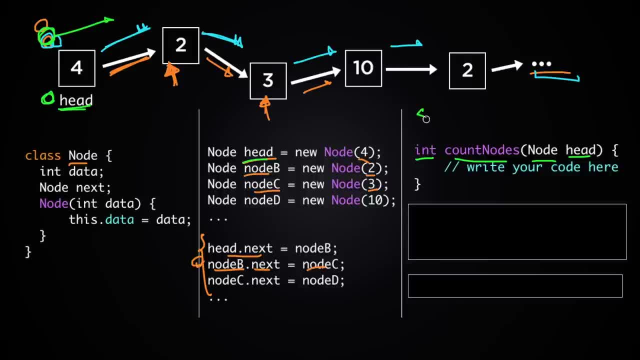 And you might wanna make it a static function, and if that's the case, you can just add the keyword static before this. If you wanna use Python to solve this problem, your function header might look like this: instead, This function is gonna be called countNodes again. 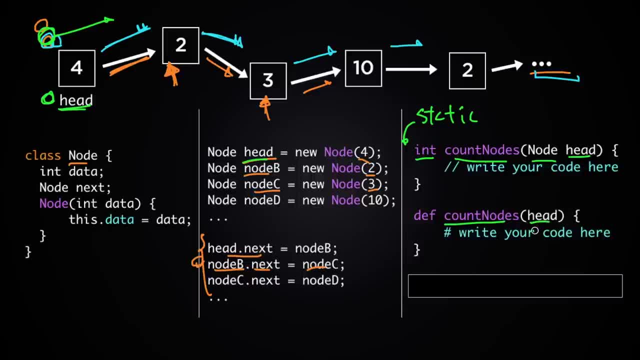 it's gonna take the head node and then it's gonna return an integer. Now, just for simplicity, you can just assume that the given head is not null And then pause the video right here if you wanna try solving this problem by yourself. 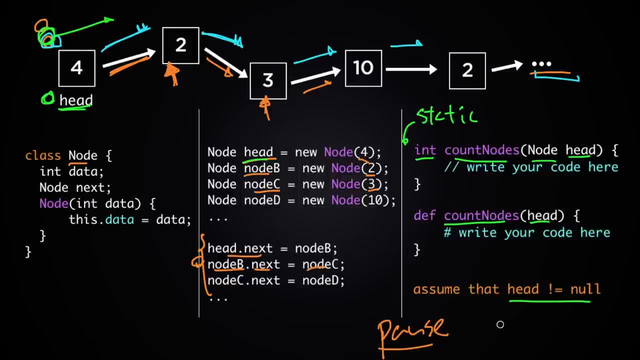 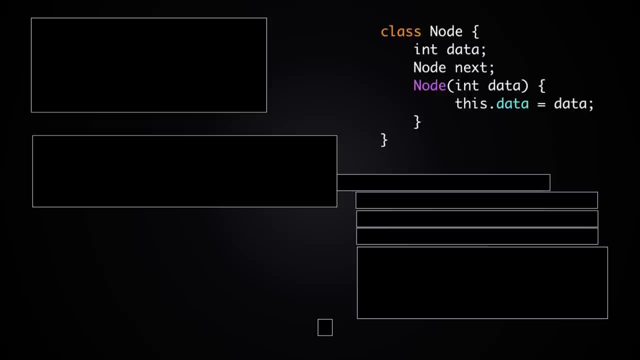 And if you were able to solve this problem, in whatever programming language you wanna use, you should post your solution in a comment below so other people can learn from it. Okay, so here's my solution. Let me first give you an idea of my solution. 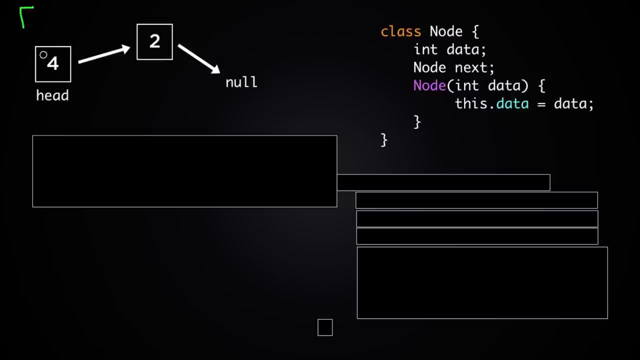 before I show you the code. So let's say you're given this linked list with the head right here. As you can see, this linked list has only two elements: this one and this one. so your function should return two And just imagine for a second. 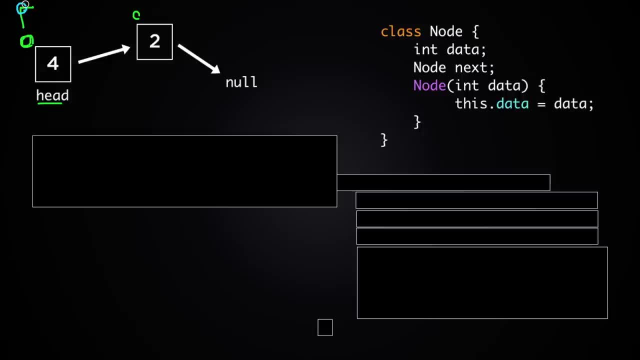 this linked list being drawn on paper. What I would do on that paper is I would point my finger at the head element, the head node, and then I would say, okay, we have at least one node in this linked list. and then I would move this finger over here. 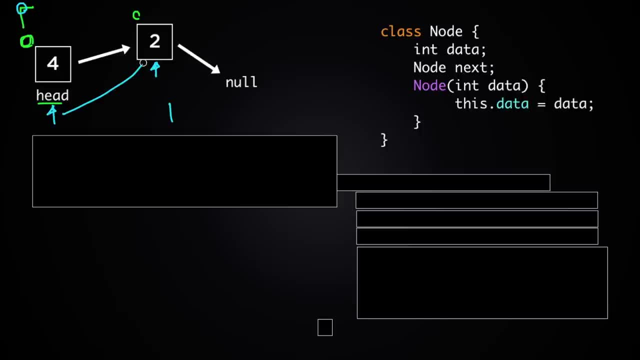 and then point at this element instead, and I would say, okay, we have at least two nodes in this linked list And at this point we'll know that this node is the last node in this linked list, because the next attribute of this node is null, right here. 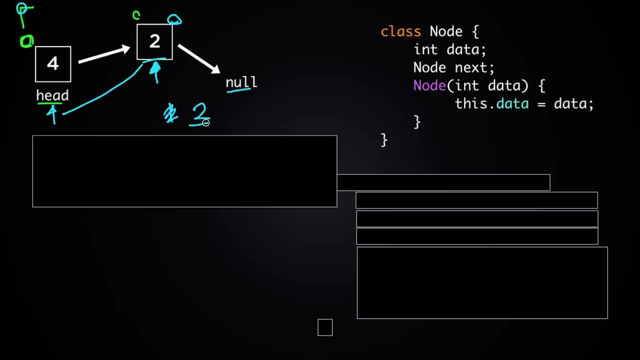 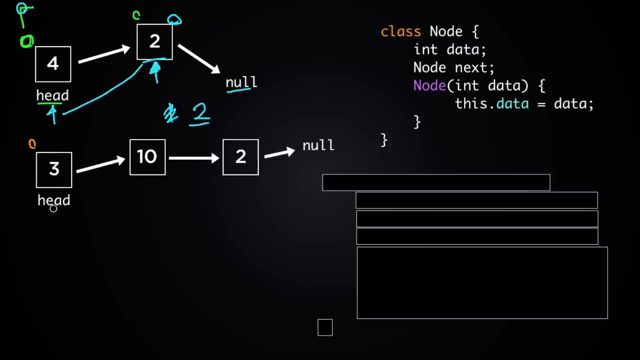 And at that point we'll just say, okay, we have two nodes in this linked list. Okay, let's take a look at another example here. We have a linked list with three nodes here and the head is this one, right here. 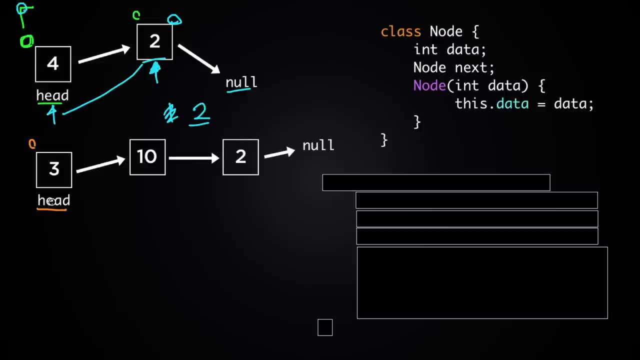 And again, just imagine this being drawn on paper. and in that case I would first point my finger at head and I would say: okay, we have at least one node here. and then I would move my finger over here and then I would say: we have two nodes at least. 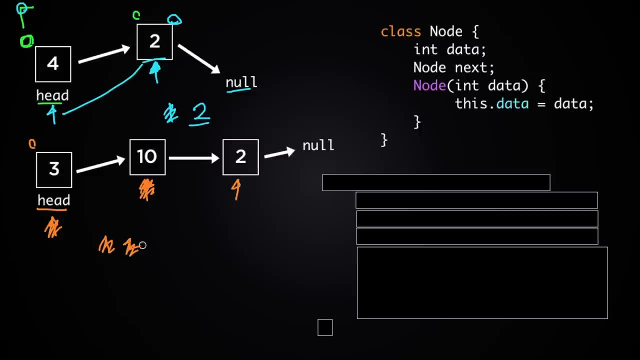 and then I would move my finger over here and then I would say: we have three nodes and at that point again, just like before, we'll know that this one, we'll know that this one is the last node in this linked list. 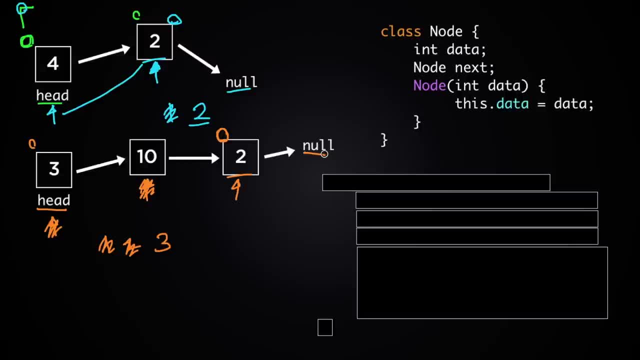 because the next node after that is just null or nothing. And let's now see how we can translate that idea into code Again. in Java we'll have a function like this, a function called countNodes, which takes the head node and returns the number of nodes in this linked list. 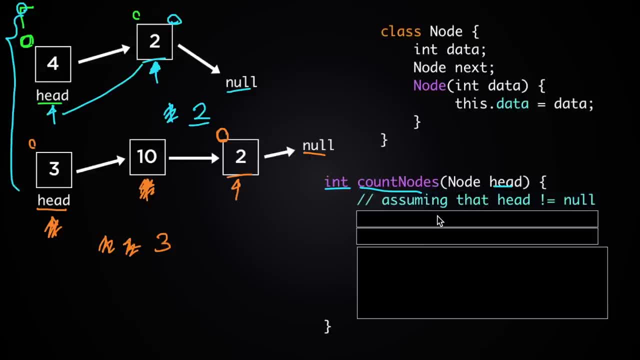 And of course we'll assume that head is not null, and then we'll define two variables: count, which is an integer, and current, which is going to be a node. And this current node. we're gonna use that to keep track of which node. 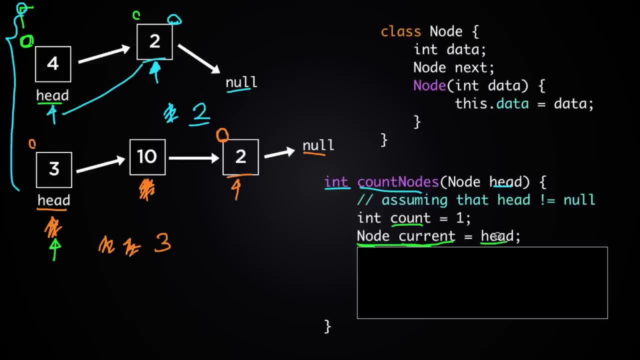 we're currently looking at. We'll start at head, of course, and then we'll use count to keep track of how many nodes we've seen so far, And then the idea is, of course, we'll move the current node from left to right. 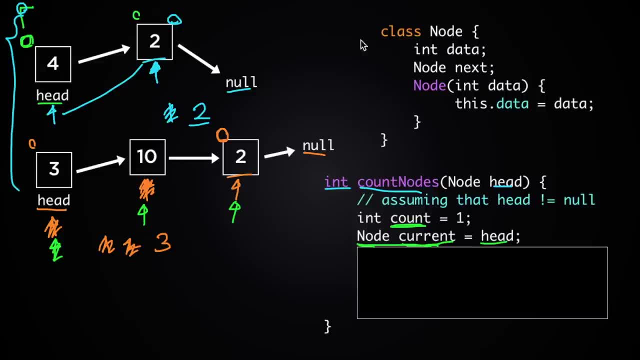 in this diagram as we increment count, And we can do this with a while loop. So here we're saying: do the following loop while currentnext is not null. So if currentnext is not null, we'll know that current is not the last node. 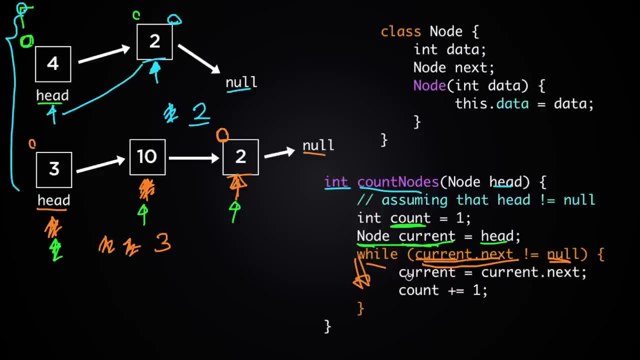 so we'll continue And then in this loop we'll update current. So if we're pointing this head right here, then current should be currentnext, which is the next node right here. So we can do that with current equals currentnext. 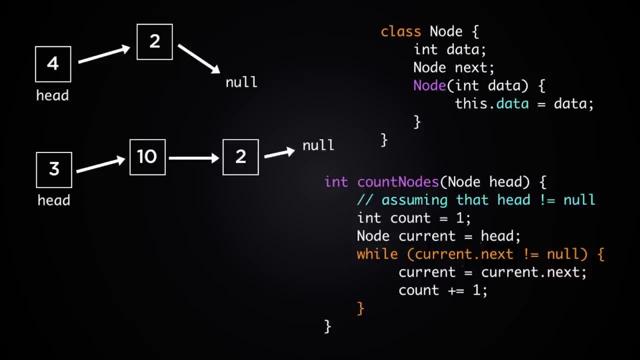 And then we'll increment count by one. Okay, let's just quickly see how this whole code works. with this example right here, Let's just say that this function takes this head right here, this node right here, and then count will become one. 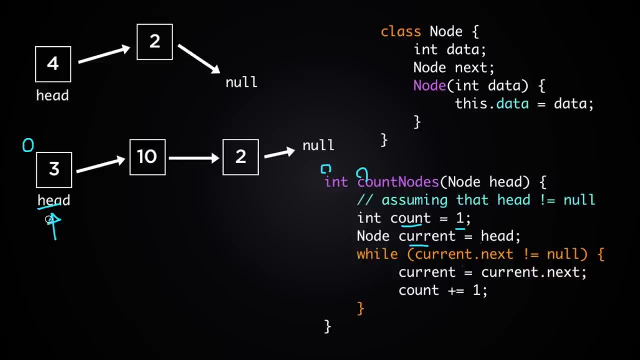 and then current will be head right here. So current will be here and then count will be one. And then we hit the while loop and then we're gonna ask ourselves: is currentnext null? Well, it's not null, so we'll continue with the loop. 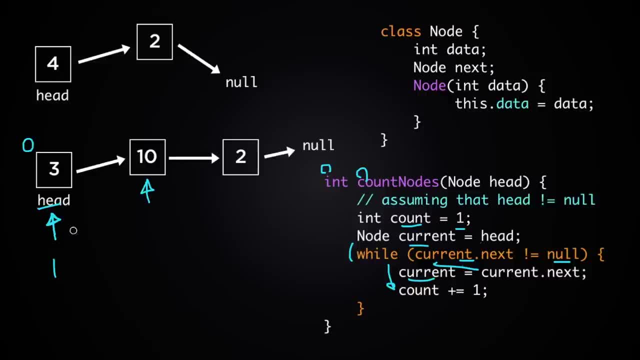 current will become currentnext, which is this one, and then count plus equals one, That means increment count by one, so count will become two, And then we'll go through the while loop again. current will be this one this time, and then count will be three. 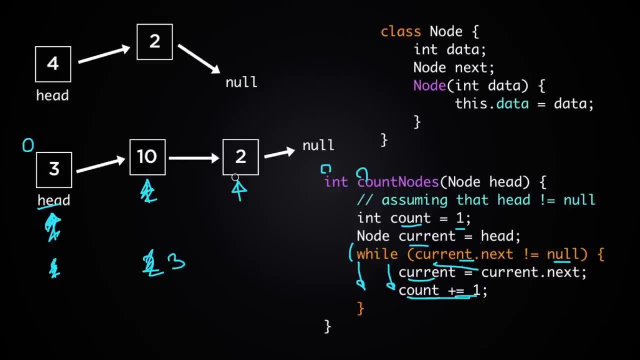 because we're doing count plus equals one again And at this point currentnext is null. so we'll stop the while loop and actually we should return. I forgot to add here countnext, So we'll return count, which is three at this point. 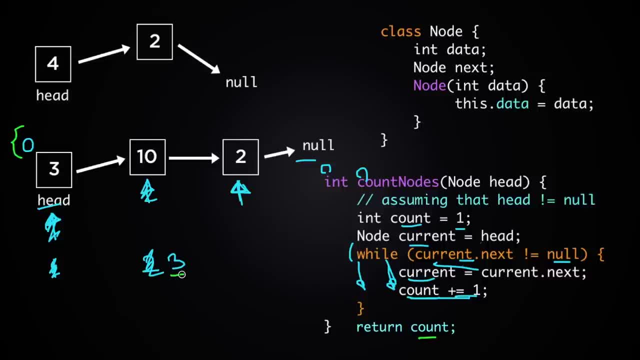 and that's the correct answer for this example. Okay, and just a quick note here. I said earlier that a linked list has connections only in one direction, from left to right in these particular diagrams, And it's true for a regular linked list. 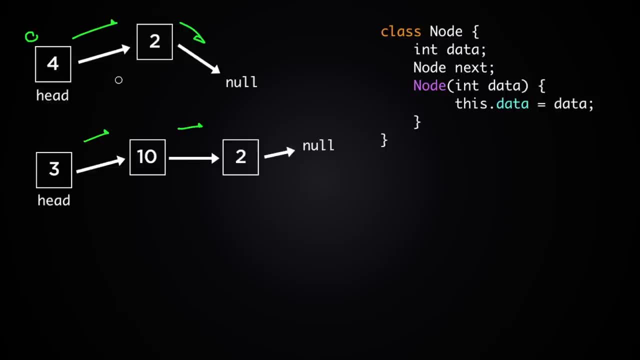 but there is something called a doubly linked list where the connection goes both ways, both forward and backward. So if we want to make a link list, we're gonna have to do this, And the way we can implement it is just by adding an extra attribute to this class. 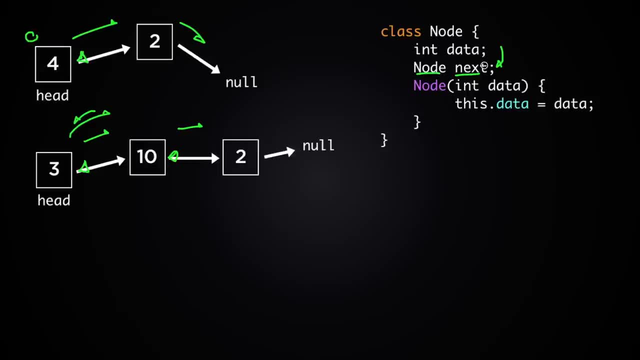 and it's gonna be just like next, which is a node, and then we can call that one, let's say preb, to show that it's a previous node. So with that, this class might look like this. I just added this attribute right here: node: preb. 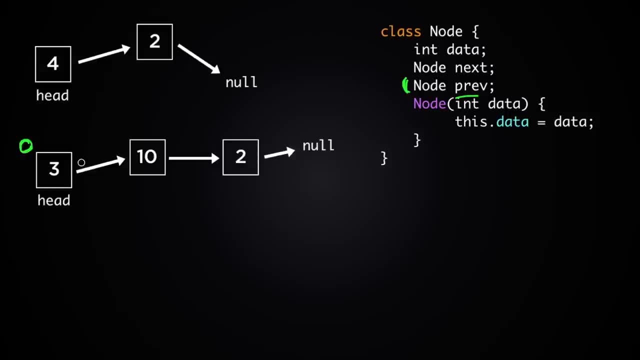 And so, as an example, if this one is a doubly linked list, and if this node is contained in a variable called, let's say, middle, middlenext will be this node right here and middlepreb will be this previous node right here. 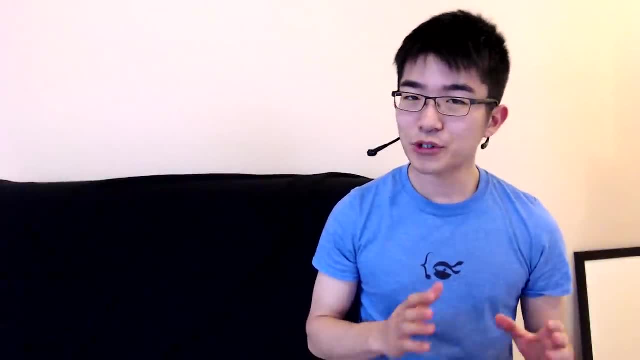 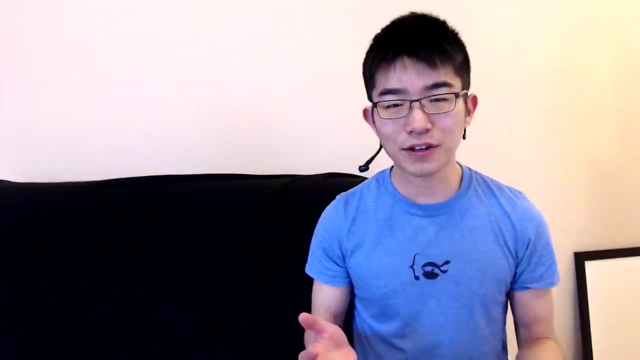 Okay, that's actually it for this video. I'm gonna cover more advanced topics with linked lists in a later video, but for now, you'll be able to find my sample code in Java and Python in the description below. And this was number five of my data structures. 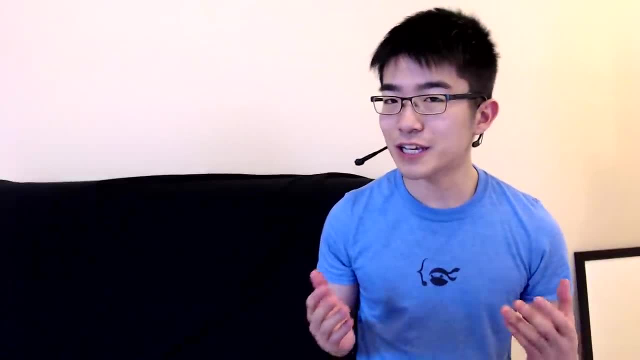 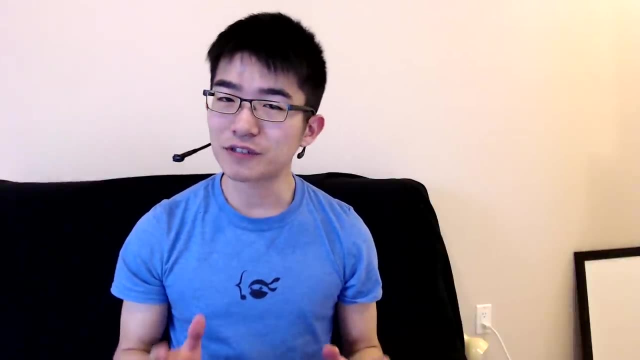 and algorithm series. You'll be able to find the entire series in a playlist in the description below, And special thanks to Brilliant for sponsoring this video. If you're watching this video as a refresher, perhaps you're looking for a way to refresh your computer science knowledge. 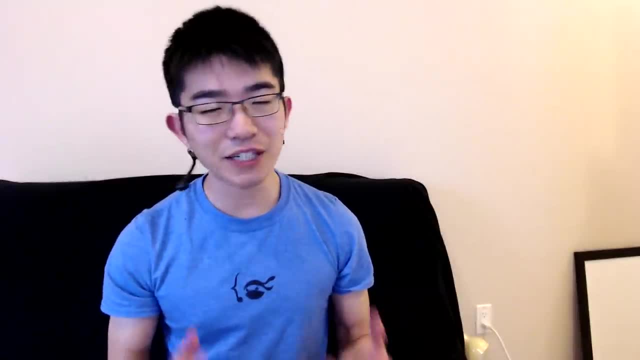 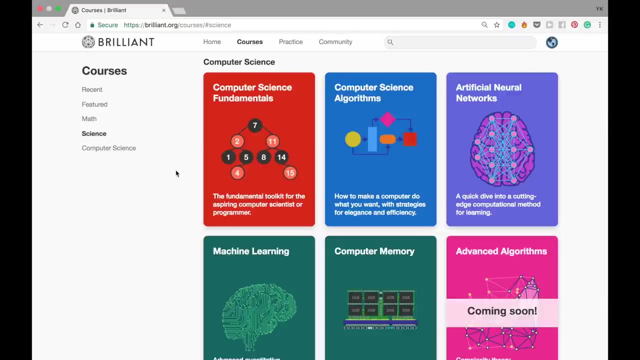 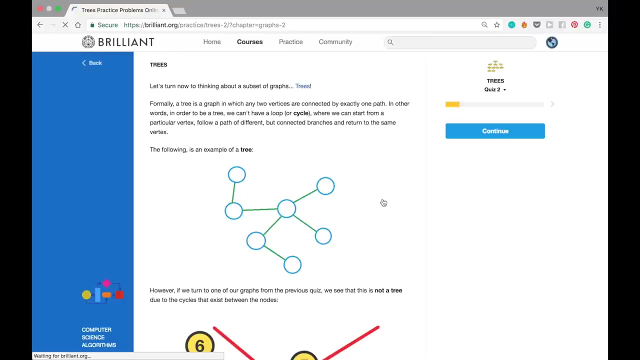 which might be a little bit rusty. Solving problems is definitely one good way to do that, and Brilliant is a good resource for finding those problems. So just as an example, let me show you a problem from their computer science algorithms course. In the graphs section they have a quiz about trees. 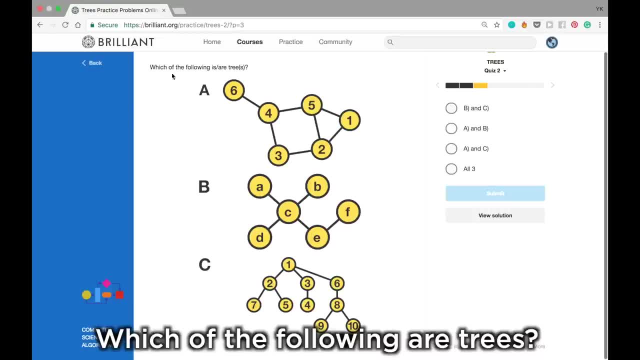 and this one says which of the following are trees: A, B and C, And the options we have here are B and C, A and B, A and C and all three. Is it all three? Actually, no, 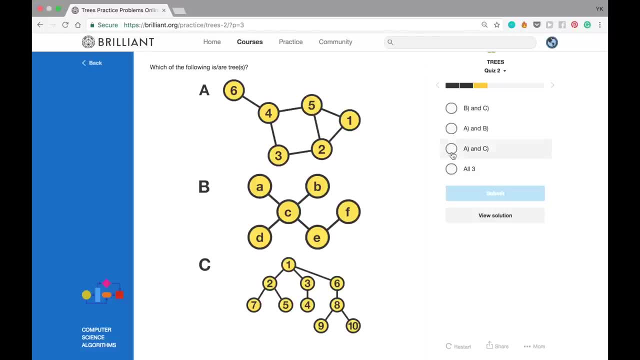 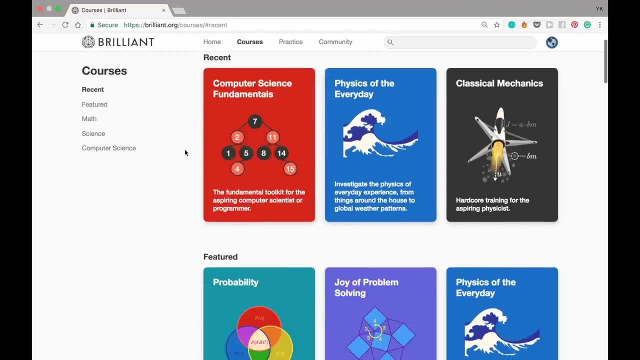 To find the correct answer and also to refresh your rusty computer science knowledge, just go to brilliantorg slash csdojo. It'll let them know that you came from here and you'll be able to get 20% off their annual subscription.